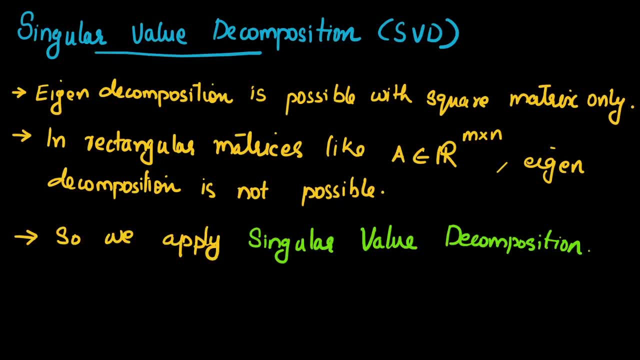 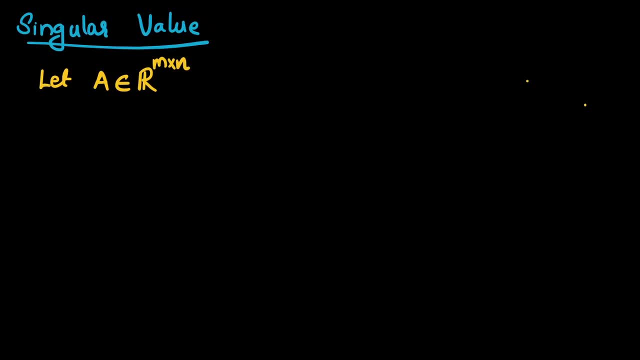 Egan, decomposition is not possible, So we apply Singular Value Decomposition or SVD. Okay, and then what is Singular Value? So, like A belongs to R, n by n, That is, A is a rectangular matrix. Consider the matrix A. transpose A. 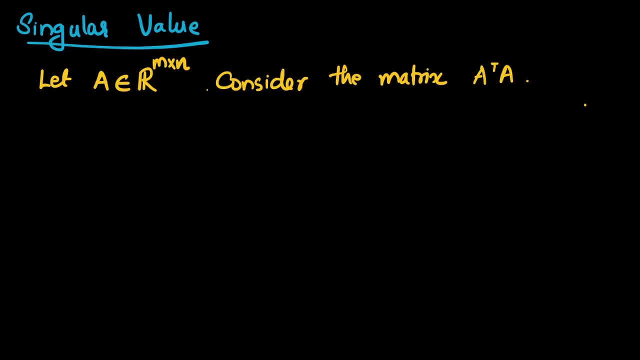 So that means take the transpose of A and multiply it with A. Okay, so that will be a symmetric m by n matrix and which is a positive semi-definite matrix. so the eigen value of a transpose a are lambda 1, lambda 2, lambda 3, etc. lambda n: the 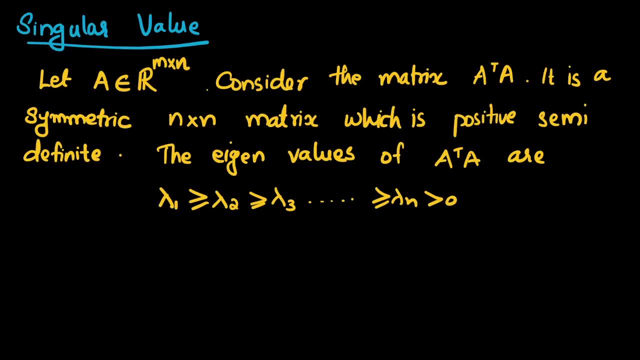 those are greater than 0 and arrange these lambda values in the descending order. that means the highest value will be lambda 1 and the second highest value will be lambda 2, like that. okay, so we have to arrange the eigen values in this order. suppose we have the eigen values 1, 3 and 8. we have to assume that lambda 1 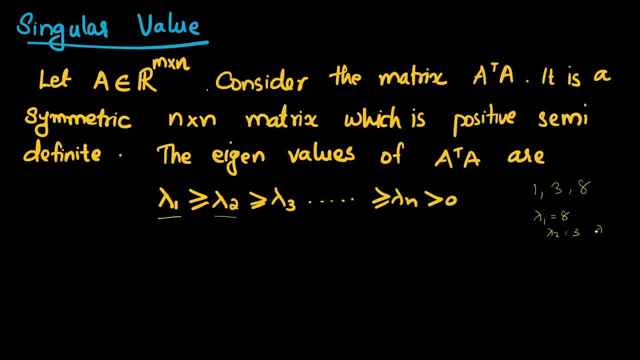 is 8 and lambda 2 is equal to 3 and lambda 1 is equal to 1, like that. so the highest value will be for lambda 1, second highest for lambda 2. like that, and take the square root of these lambda values. we represent it as Sigma. okay, so? 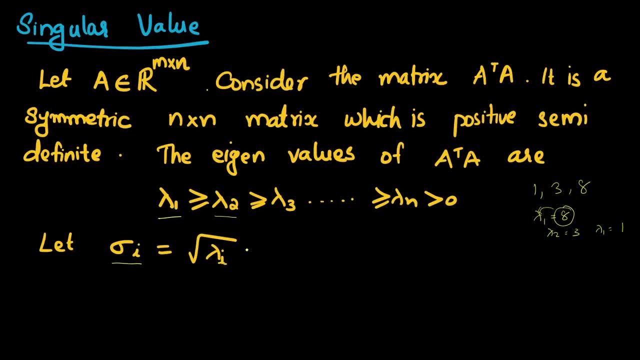 Sigma I is equal to square root of lambda I. that means Sigma 1 is square root of lambda 1 and Sigma 2 is equal to the square root of lambda 2, and so on, and we call this Sigma value as the singular value of a. okay, so this Sigma is called the singular value. 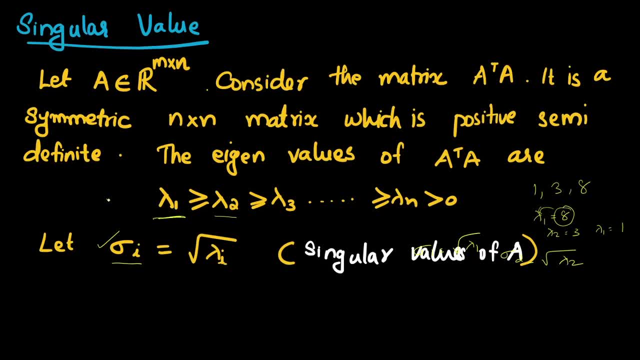 of a. this lambda is actually for a transpose a. okay, so this is: this is the eigen values of this metric. the metric matrix a transpose a and Sigma is actually the singular value of the matrix a. okay, so instead of eigen value, we are going for the singular value in. 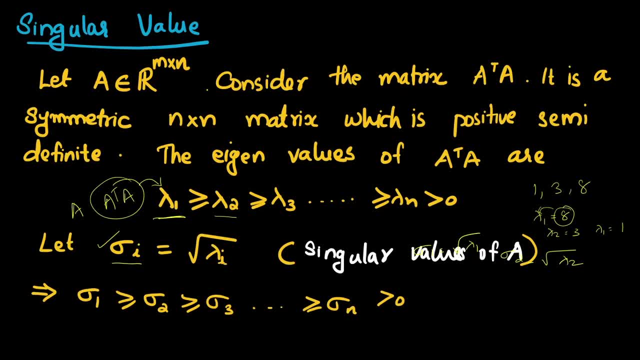 this decomposition. okay, so then, as Sigma 1 is greater than or equal to Sigma 2, greater than or equal to Sigma 3, that relation will be kept, even after we are taking the square root. okay, so this relation will be kept and this values are greater than or equal to Sigma 3. 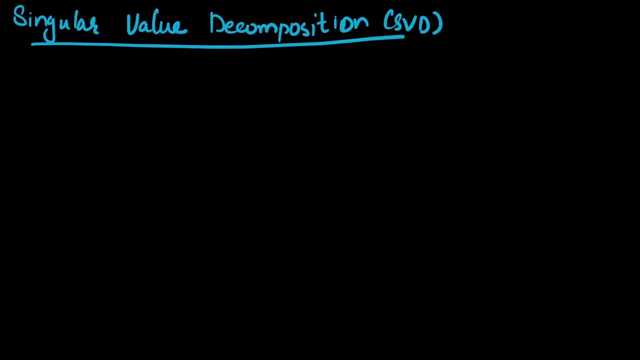 zero. okay, and these sigma values are the singular values. and how do we do this singular value decomposition? let a be an m by n matrix and assume that its rank is equal to small r. the singular value decomposition of a is: a is equal to u. sigma V transpose: okay, so this is the form of singular value decomposition, SVD. 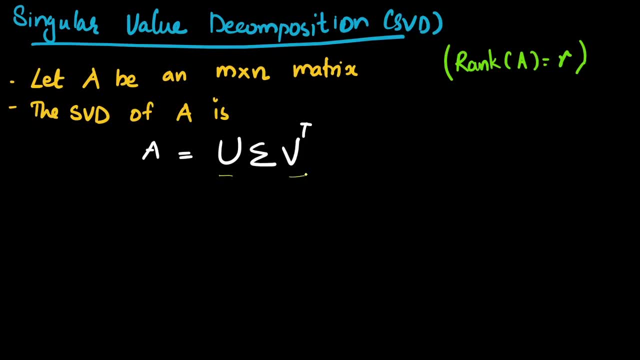 and U and B are the orthogonal matrices, okay, made up of the Hagen vectors, and Sigma is the diagonal matrix, made up of the sigma values. okay, these sigma values, Sigma, one, Sigma, two later. okay, all the other elements are zeros. so that is water, Sigma, okay, so these three, so a can be decomposed. 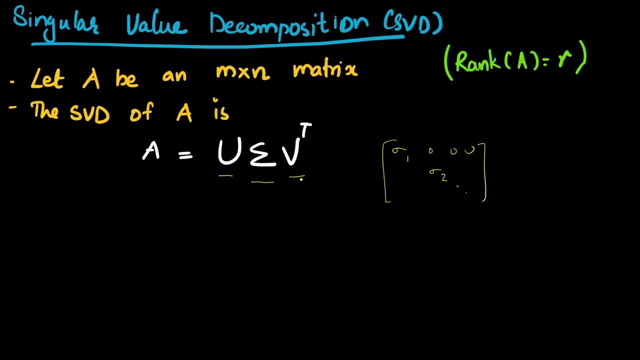 in f- water and p- air form of these three matrices, u, sigma and v. transpose. and let's see what are these matrices: u, sigma and v. okay, so where u is an m by m orthogonal matrix. okay, so remember, our matrix size is m by n. rectangular matrix size of a is m by n. and here u is an m by m orthogonal matrix. 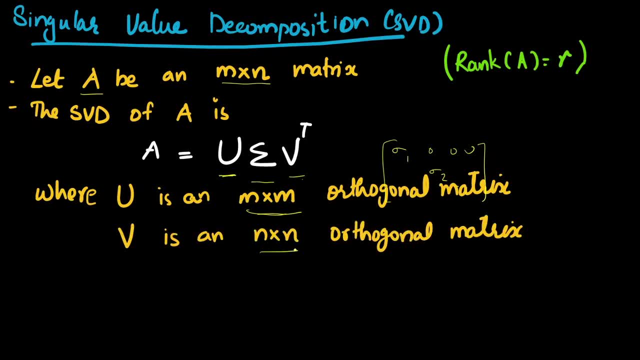 and v is an n by n orthogonal matrix and the sigma is an m by n matrix, where diagonal elements of first r rows are singular values of a and the remaining entries are zeros. okay, so why we call it as r? because its rank is labeled as r. so the rank of the matrix a is r. so the first n, first r. 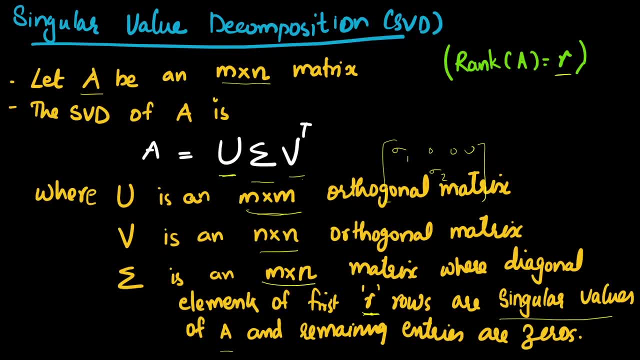 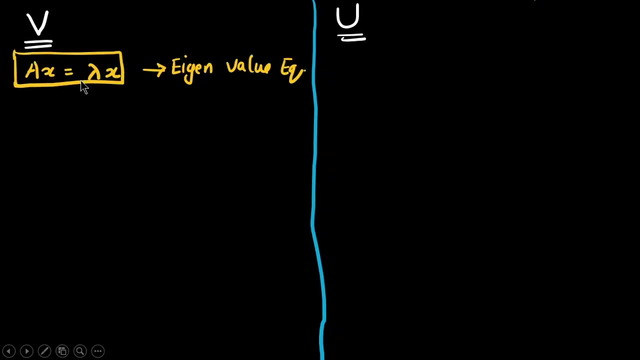 rows will contain the singular values and this remaining will be zeros. okay, and the size of this matrix is m by n. so so please make note of these dimensions. okay, u is m by m and v is n by n, and sigma is m by n. and how do we calculate u and v? so first we can go for v, so we take the. 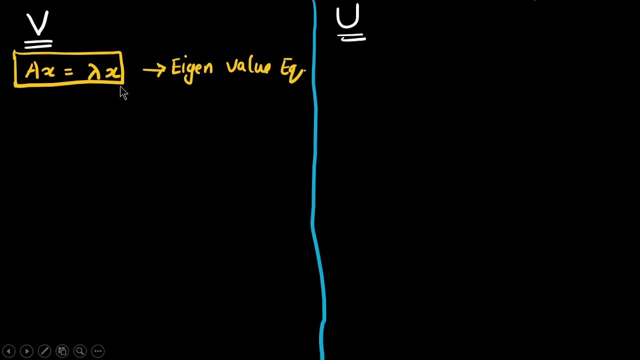 eigenvalue equation, ax is equal to lambda x. okay, so keep this equation in mind. and if a is equal to m by n matrix, and what will be a transpose a? okay, a transpose a will be n by n matrix, because a transpose is n by m and this a is m by n. so when? 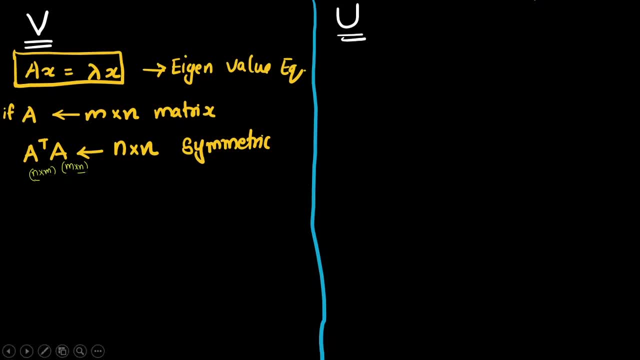 we multiply it, we get an n by n matrix. okay, it's a symmetric matrix and we apply this: a transpose a in place of this a in this eigenvalue equation. so we will get a transpose a into x is equal to lambda x and where x is the eigenvectors. 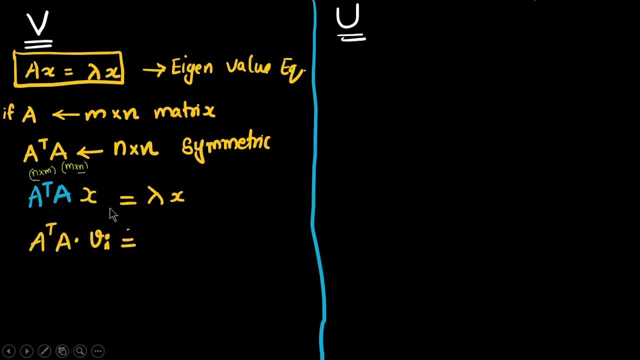 and lambda is the eigenvalue. okay, so, um, here we uh, we rename this x as vi. okay, in order to uh differentiate this v and u matrices. so we take it as vi. a transpose a into vi, and so this vi is actually the eigenvector of this matrix. okay, a transpose a. 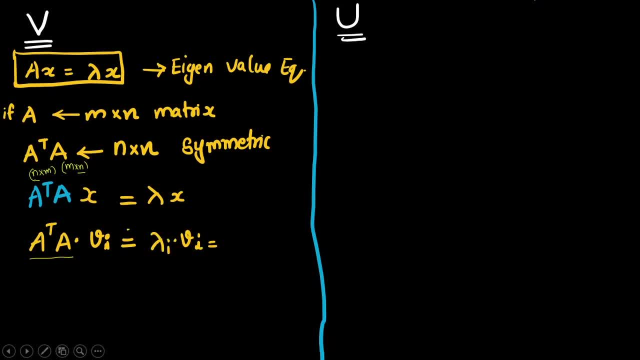 okay, so vi is equal to uh. instead of lambda. we are writing lambda i into vi, so lambda can be replaced with the sigma value: sigma i, square. okay, so sigma is sigma is actually root of lambda i, so we use the square here. lambda, sigma i, square vi. okay, so from this uh, we have to calculate uh, vi. 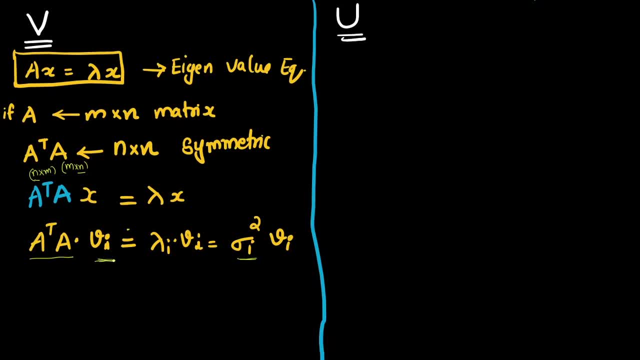 so for every sigma value we have to find out the vi vectors, okay, eigenvectors, corresponding to each sigma value. okay, and this: we will get v1, v2, like that, and arrange them in in in columns and we will get the vector or the matrix v. okay, so vi's are the pairwise, orthogonal and orthonormal. 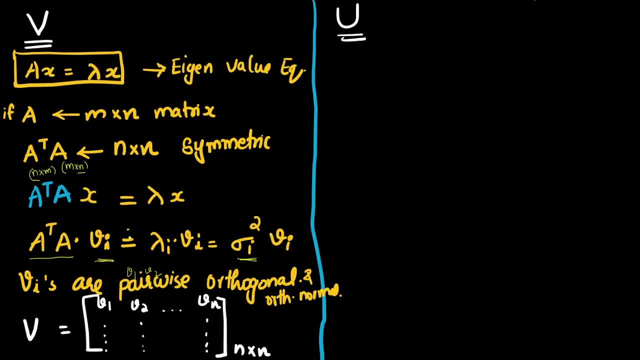 matrix vectors like this: each column represents each eigenvector- v1, v2, etc. vn. okay, so first column represents v1, second column represents v2, third column represents v3, and so on, and the last column will represent vn. so finally, this will be an n by n matrix. okay, so we we start with a rectangular. 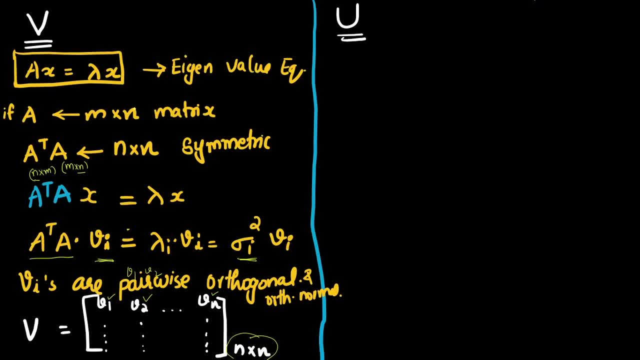 matrix and we convert into, we make it into a square matrix by taking its transpose and multiply it with itself. okay, so then we got an n by n matrix and find out the eigenvectors of this matrix and we will get the corresponding vector, v vectors and finally the matrix v. 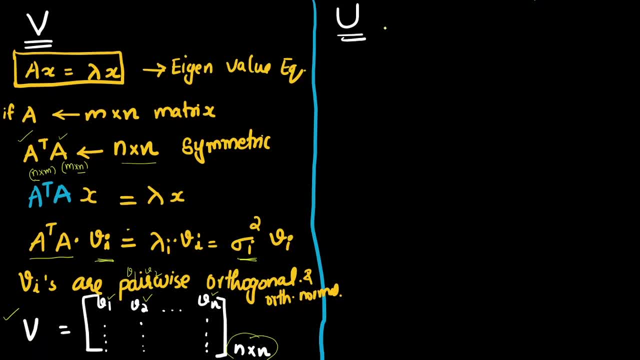 okay, so that is an n by n matrix. and now we have to go for m by m by n matrix, u. okay. so how do we do we multiply with with the a transpose so that we give you an m by n matrix? okay, so a is an m by n matrix. is a into A transpose, is m by M and find the eigenvectors of a into. 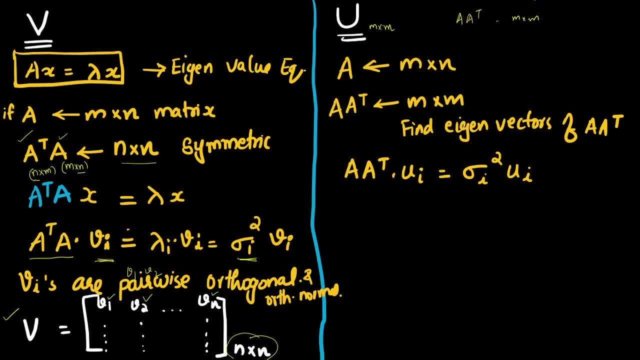 A transpose- this is equal to A- into a transpose: u i is equal to sigma i square u- i. so here we, the eigenvectors are represented with the UI. okay, then find out the UI values and write it in columns: u1, u2, like that. so first color represents u1, second. 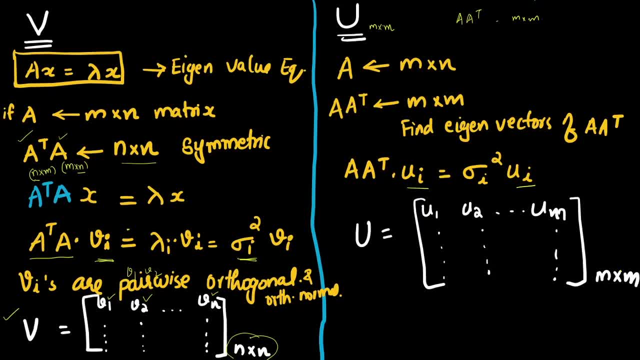 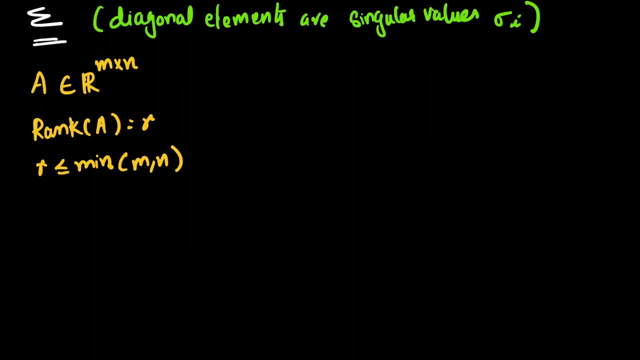 color represents u2 up to UM. so this will be an M by M matrix. okay, so that is V, that is U and okay now. Sigma is the diagonal element and the it's a diagonal matrix whose diagonal elements are the singular values, Sigma values. okay, then it will be written like this: Sigma 1, Sigma 2, etc. Sigma R and these are the. 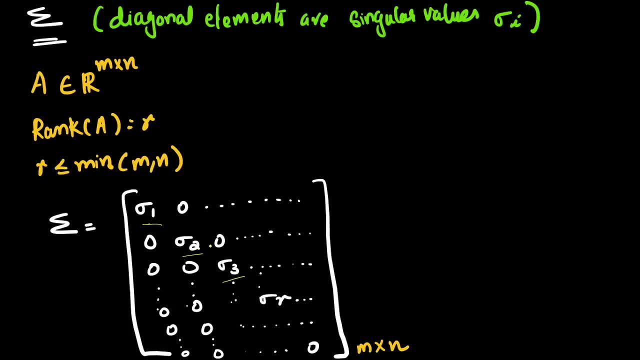 diagonal elements are the singular values and all the other values are zeros and the dimension of the space is V, that is U, and now Sigma is the diagonal element and the diagonal matrix is M by M. okay, then we can see an example: find the singular value of. 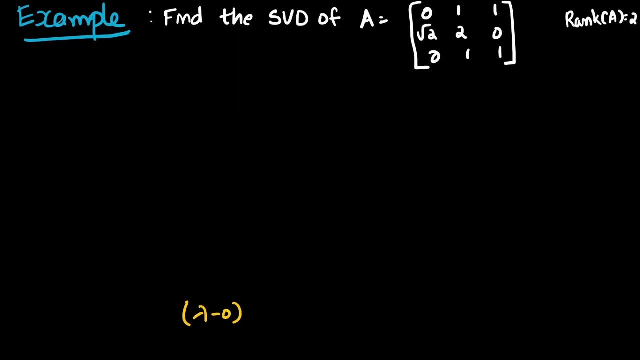 singular value, decomposition of a. so this is the matrix and the rank of the matrix is given as 2. okay, so we find out a into a transpose- this is a- into a transpose equal to this matrix. and we are to find out. it's a. again, we are to find out, it is a neue. we are to find out where thisới the. 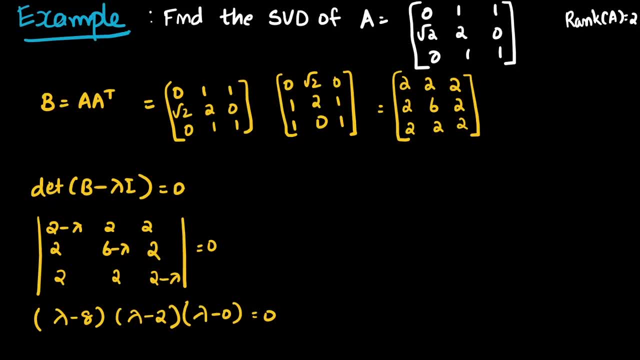 gender value. yes, there is commune somewhere, and that's where the Beetle will be equal to zero, because cosa Essexлем in that road is equal to zero, but there's still an L. that is the�동ial: ♥ 다양한óg. it will be written like luars �. so, being the Mean handedogle, give a greedy and find out what is ti- Principle values- into the finite 코 a, tissues b, the bereavement table, And we then take the elimination declaration. We finally we get it like this: so the lambda values can be Parking. the lambda values can be zero, two and 8. okay, So the first lambda two will be L is r 8 and the 2 is 0. So the Sigma values can be written like this: Sigma 1 is 2, root 2, that means it is root 8, and sigma 2, banh two root and one isjet 1, That means it is 0 or root 20.. 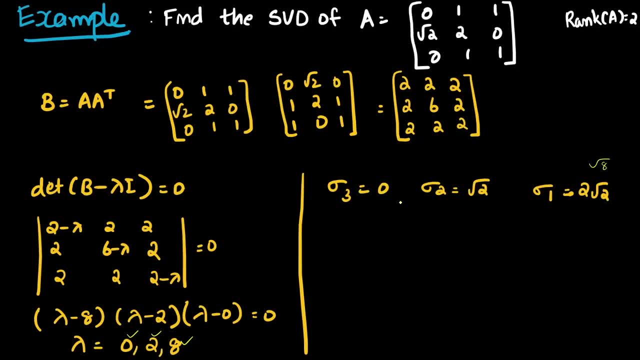 2 is root of lambda 2 and sigma 3.. So these are the sigma values And we can find the eigenvectors for these lambda values. Okay, As described previously. So the u1 values we will get, like this: u1, u2, u3, like this: 1, 2, 1.. Okay, u1 is 1, 2, 1.. u2 is minus. 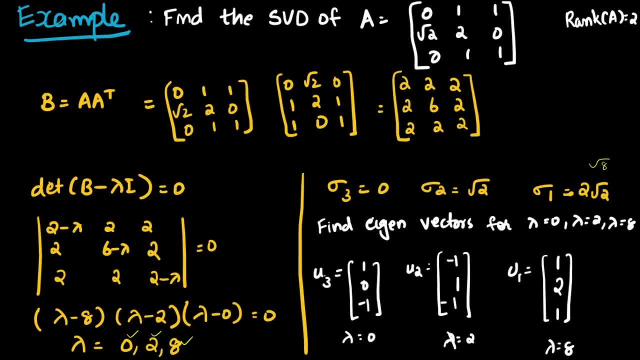 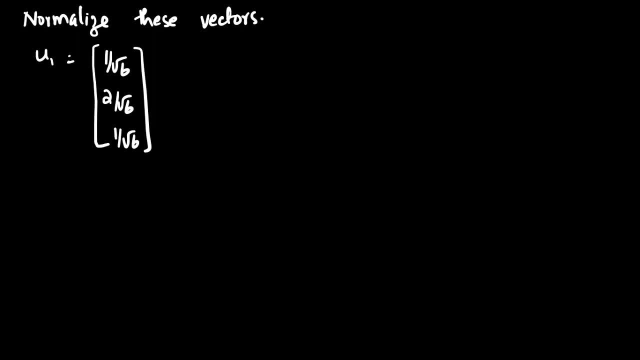 1, 1 minus 1.. And u3 is 1, 0 minus 1.. Next we have to normalize these vectors: 1 by root 6, 2 by root 6 and 1 by root 6.. So how do we normalize a vector? So if we have a vector, 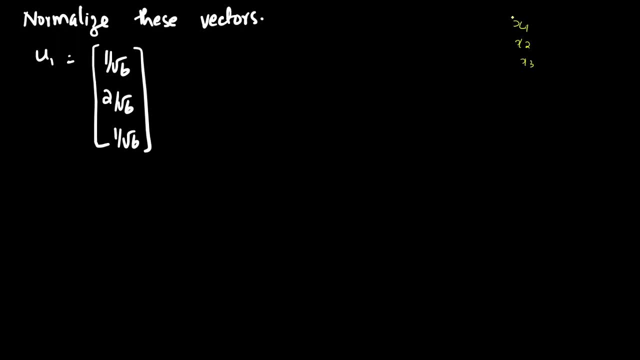 like this: x1, x2 and x3. how do we normalize? First of all, we have to find out the square root of the sum of squares x1.. So x1 square plus x2 square plus x3 square. Okay, So in order to normalize it suppose 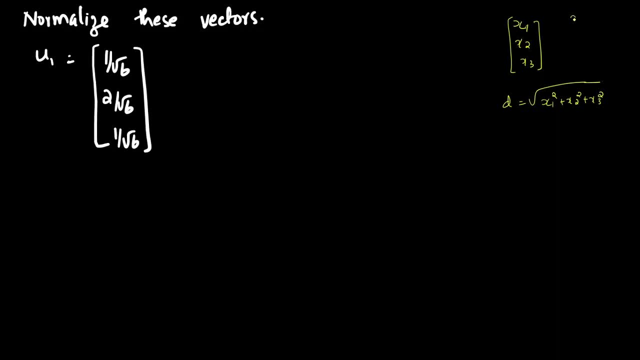 this is d. Okay, So what we have to do? we have to multiply, divide it. Every element has to be divided with this d. Okay, So this will be the normalized vector, Right, Okay? So, similarly, here, the u1 was 1,, 2, 1.. So we find out d value as root of. 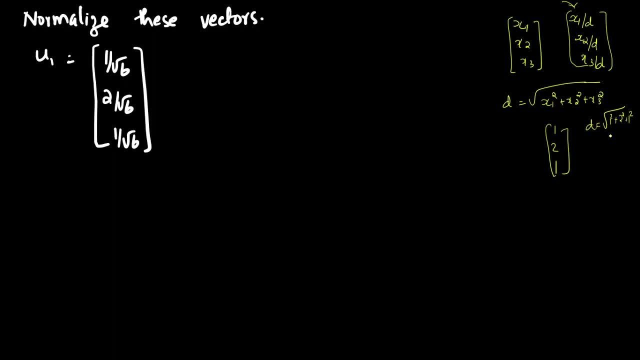 1 square plus 2 square plus 1 square. So that is is equal to root 6.. Okay, We have to divide every value with root 6 so that it will become normalized Like that. Okay, what happened here? one by root six, two by root six and one by root six. so similarly u2 and u3. 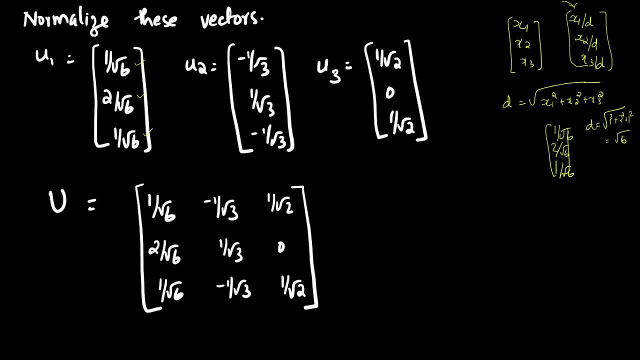 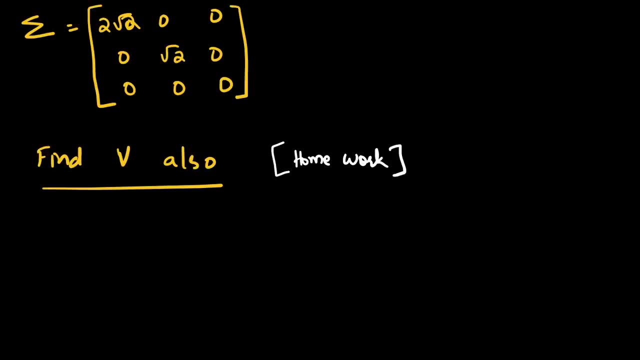 will be normalized and finally we'll get u like this: arrange it in order. so this is u1, the first column is u1, second column is u2 and third column is u3. okay, and in the same way we can find out v also, and the sigma is written like this: it's a, it's a three by three matrix. okay, and then this: 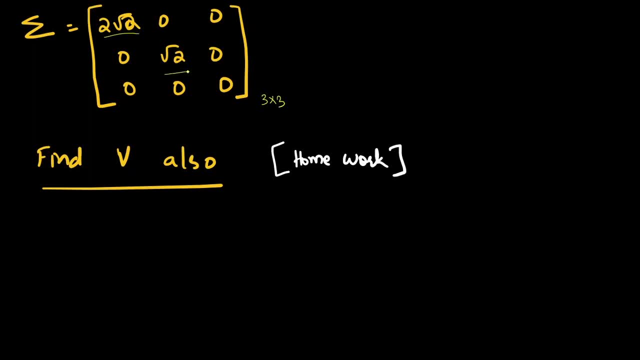 is the first sigma one, value sigma one. this is sigma two and this is sigma three. okay, this is. and find the value of v also. okay, so when you calculate, you will get v as this. okay, this is another example for a rectangular matrix. follow the same procedure and find out the answers. okay, so sigma will be like this: root six. 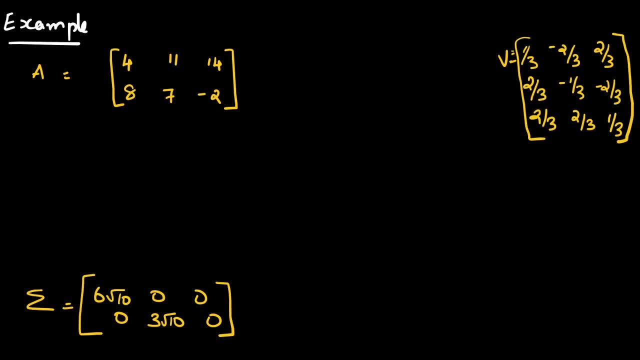 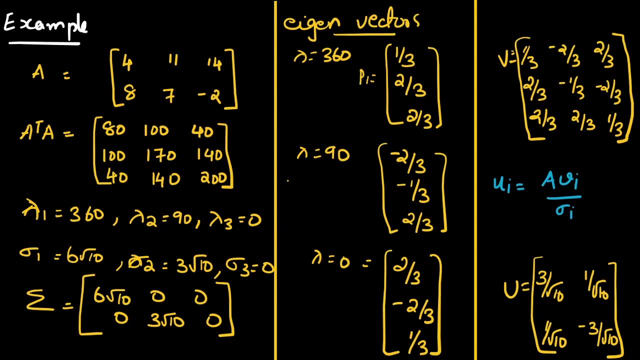 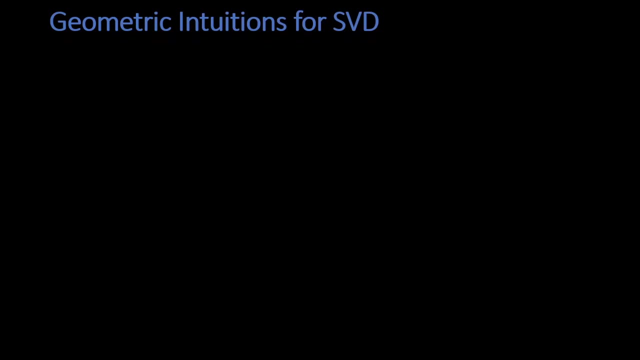 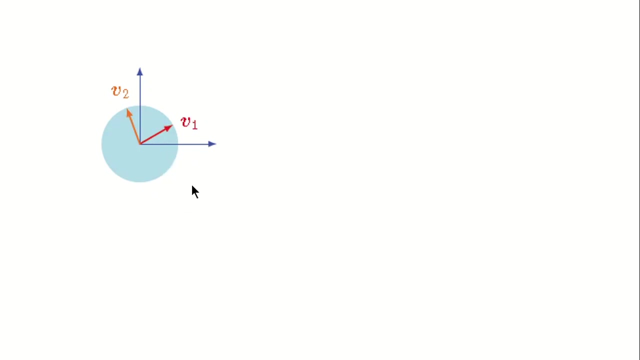 six root ten, three root ten, like this, and v will be this one and u will be this one, okay, so you can do it on your own and to compare the answers. and next is the geometric intuition of the singular value. so these are the, this is the vector space we have, okay, and when we apply the v, transpose uh, they will change uh there.